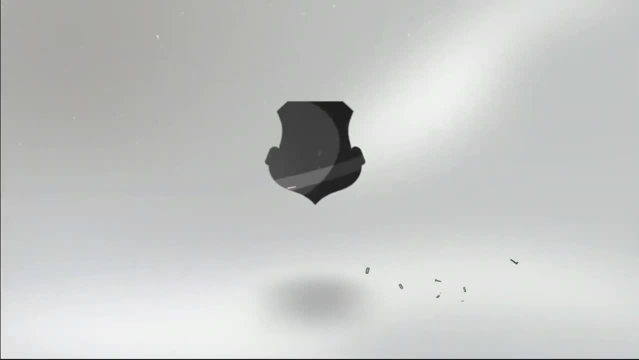 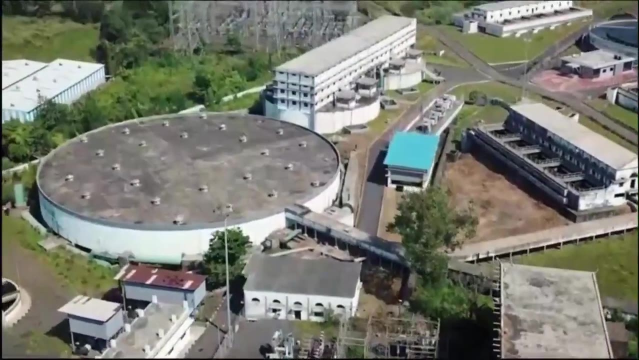 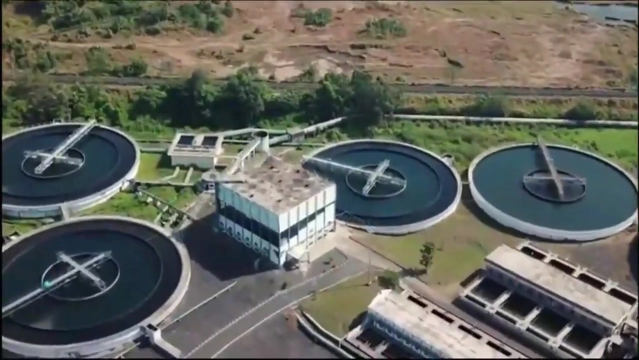 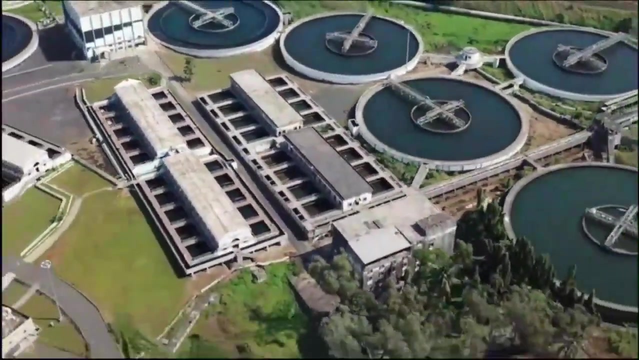 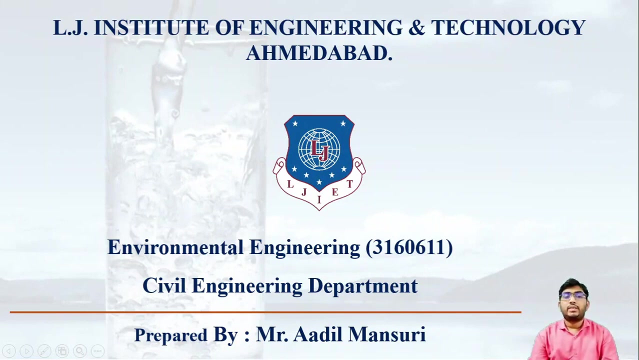 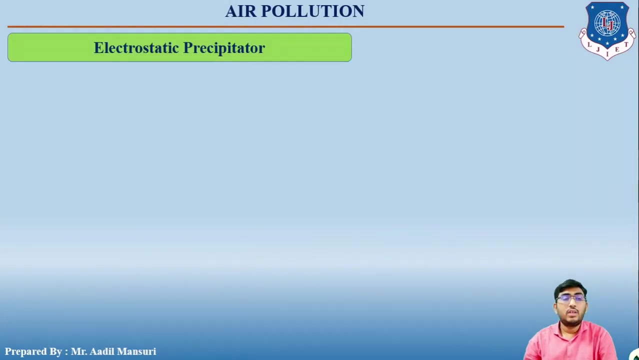 Welcome back students to the video lecture series. I am Adil Mansoori from Civil Engineering Department of LJ Institute of Engineering and Technology. So let us now move ahead with the next topic. So next is electrostatic precipitator. So the picture shows you electrostatic precipitator. 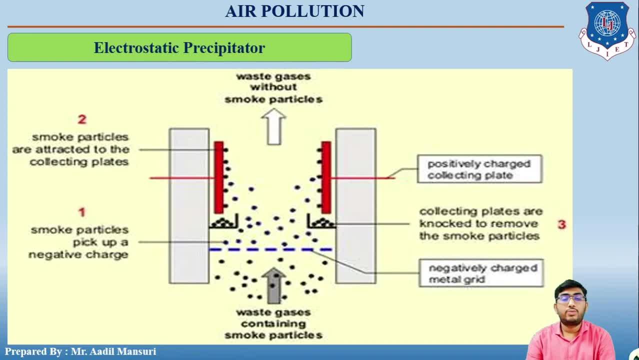 So electrostatic precipitator is one of the most widely used devices for controlling particulate emission at industrial installations, ranging from power plants, cement and paper mills to oil refineries, And in most of the cases, the particulates to be collected are byproducts of the combustion. 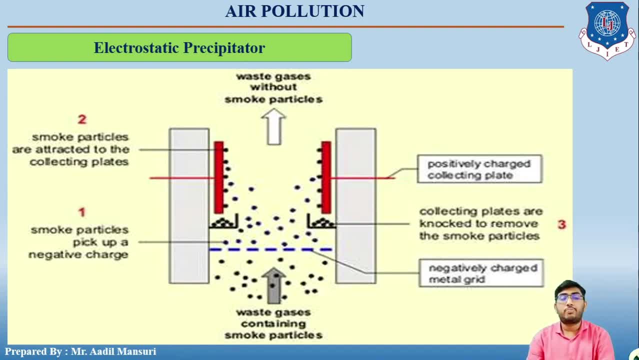 Electrostatic precipitation is a physical process by which particles suspended in a gas stream are charged electronically and, under the influence of electrical field, separated from the gas stream. For industrial applications, vertical plates exposed to horizontal gas flow are normally used, And in this type of collectors 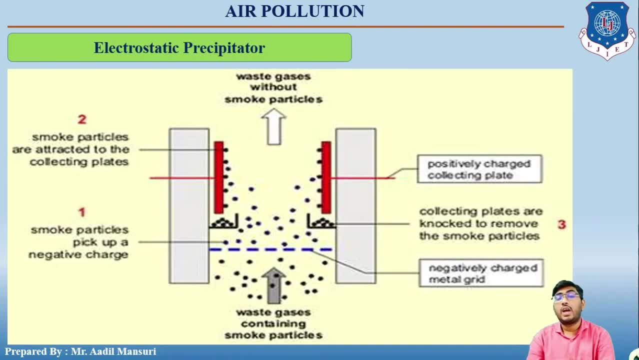 the gas flows between two parallel plates, between which are suspended a number of vertical wires held in place by weights attached to the bottom. Okay so these wires form the discharge electrodes, while the vertical plates from the collection electrodes. Okay so, talking about the advantages it has, the particles as small as 0.1 micrometer can also be removed. 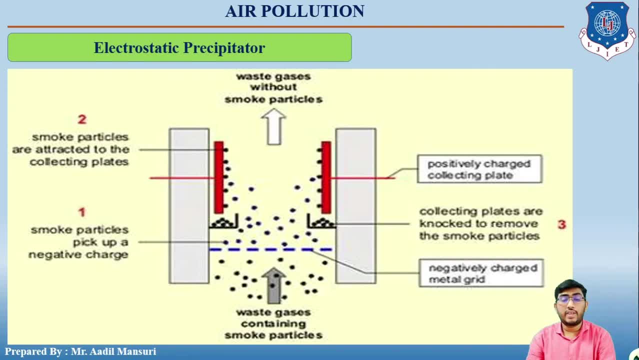 Okay then higher collect Collection efficiency, then power requirement is less, then large gas column can be handled okay and pressure drop is less. that is 0.25 to 1.25 centimeter of water and can remove tar and acid mists. 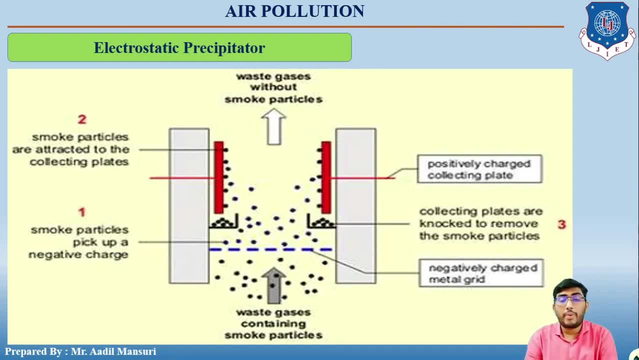 Okay then it has an ability to operate over a wide range of conditions, even temperatures of up to 800 centigrade and pressures of up to 50. atmospheric pressure can also be treated. Okay, and pressure drop is one month and there is an opportunity to Okey. 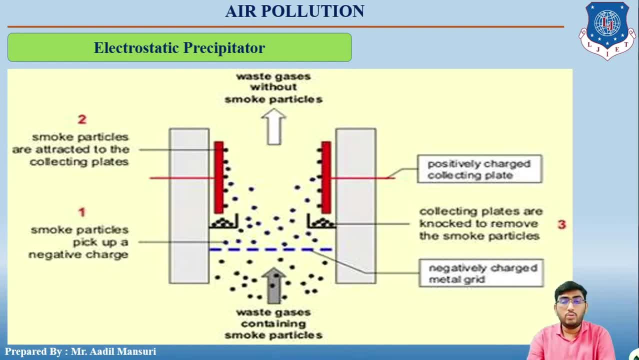 And treatment time is very negligible. that is point one to 10 seconds. Okay, and talking about the disadvantages, it has high initial costs. Large species hurricane on high voltage equipment necessitates special safety precautions. right, There are possible explosion hazards during collection of combustible particulates or gases, and collection efficiency reduces with time. 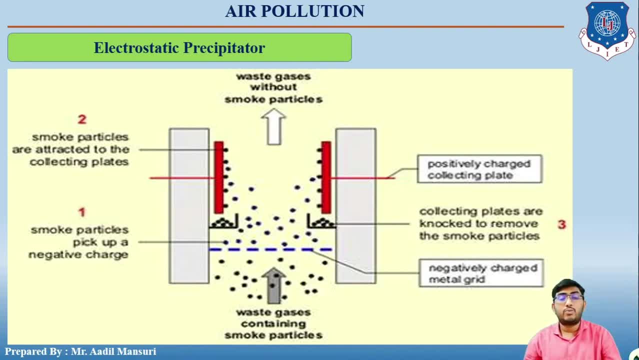 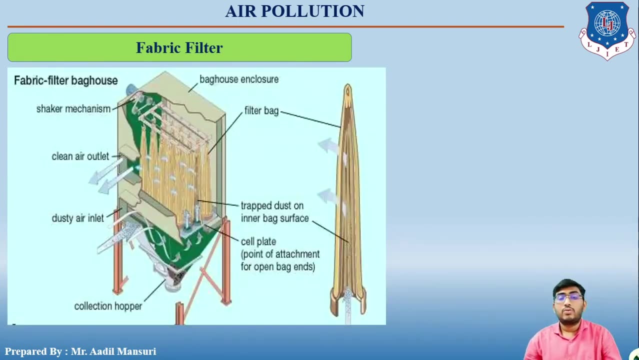 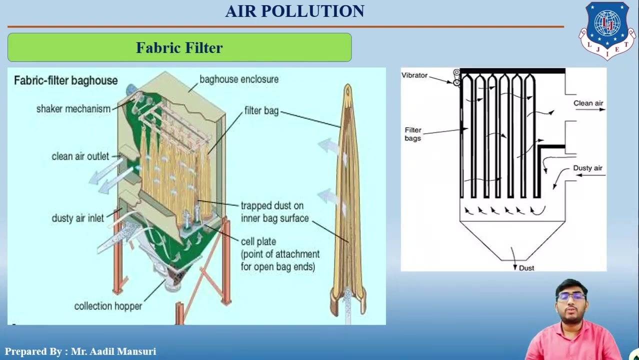 then sensitivity- sensitive to variable dust, loading is driving primaryantly- and flow rates. okay, so these are certain disadvantages, so moving further. next is fabric filter. okay, so fabric filter, or it is also known as the bag house, right, so fabric filter consists of a tubular bags or an envelopes suspended or mounted with open cells in such a way. 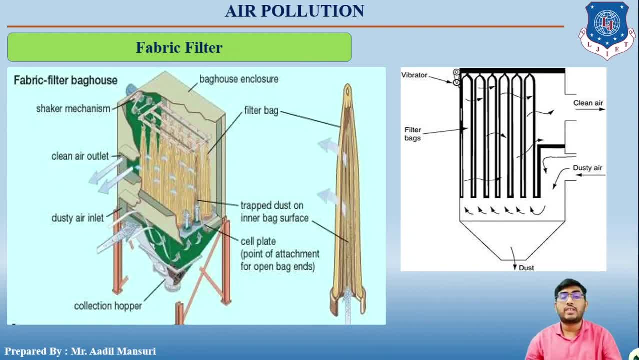 that when dirty gas pass through it, the particulate matter is arrested on the inside fabric surface of the bag. okay, and the whole system generally known as bag house consists of number of such bags. you can see in the picture right. the upper ends of the bags are closed, while 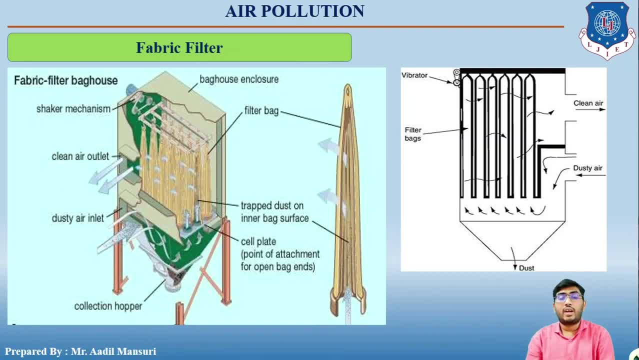 the lower ends are attached to a hopper and where also the inlet of the flue gas is located. okay, and the upward moving gas? the upward moving gas drops out particulate matters in these bags, which settle down into hopper and cleaner gas goes out through the. 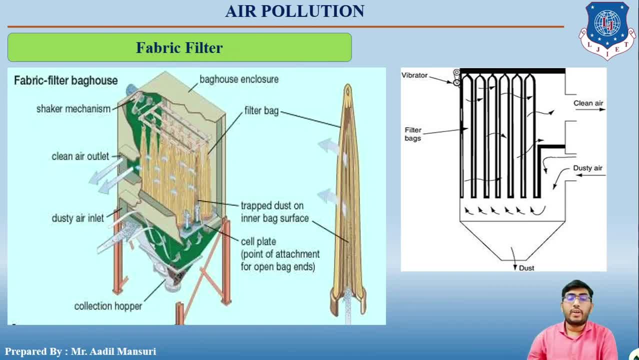 fabric filters. the framework is provided with an automatic shaking devices for cleaning the bags of the collected dust. okay now, the normal velocities at which the gas is passed through the bag is 0.4 to 1 minute- sorry, 0.4 to 1 meter per minute, and the air to cloth ratio is one. 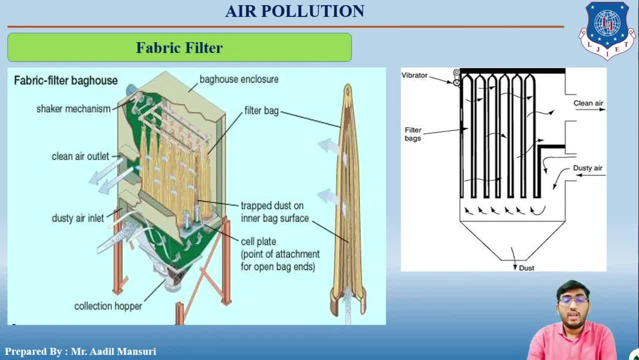 of the important parameters in designing of these filters. in the low ratio bags, the air to cloth ratio is between 7 to 25 mm per second, while in high ratio bags, this is value is 25 to 50 meters per second. okay, talking about the advantages, uh, high collection efficiency, about 99 percent collection. 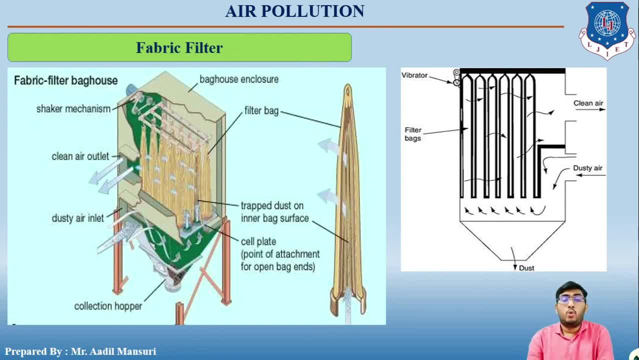 and disposal of particles in dry form. then low pressure drop. fine, then simple construction and then nominal power consumption. okay, so these are the advantages. talking about disadvantages, uh, large size of equipments are needed, right then. operational limitations for process temperatures are higher than 285 degree centigrade. high initial construction cost, then operational limits at high. 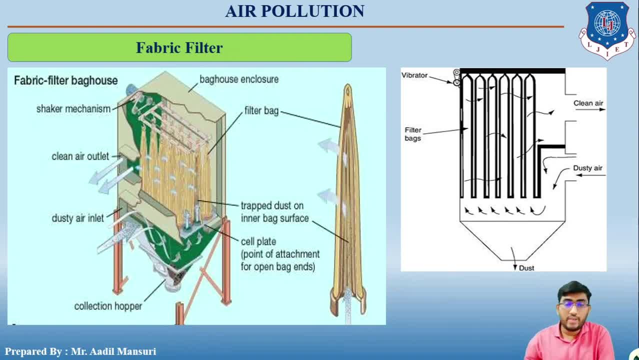 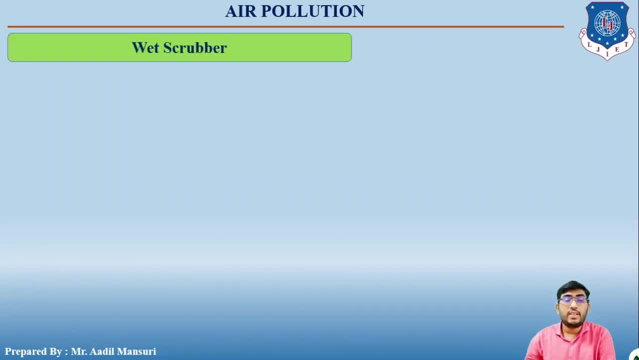 humidity, and the fabric is also liable to chemical attack. okay, so let us now move towards the next phase: wet scrubber. so a wet scrubber is a device which utilizes a liquid to assist in the removal of particulates from the carrier gas stream. they are mixed phases of gas and liquid. the object of 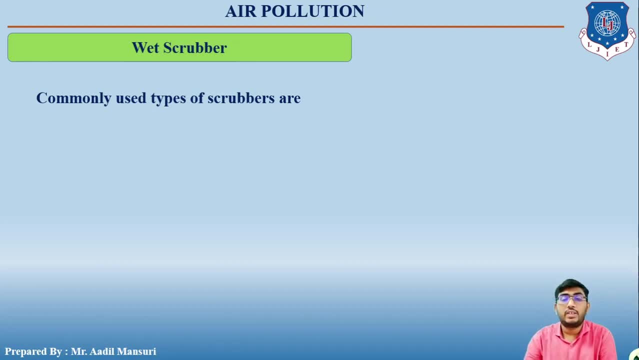 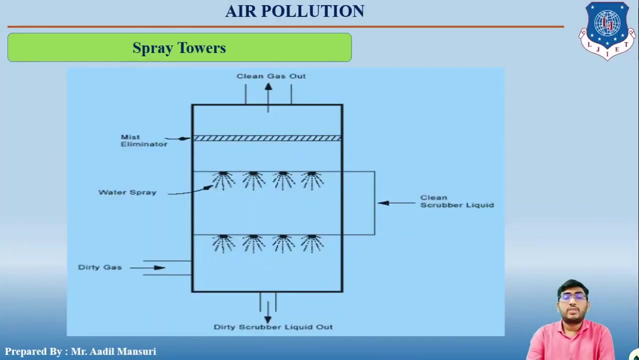 the scrubber is to transfer suspended particulate matter in the gas to the scrubbing liquid, which can be readily removed by the gas cleaning devices. okay, so common types of scrubbers are spray towers, bag bag towers and cyclone scrubbers. okay, so let us have a look at each of them. so, spray towers- you can see the picture. so the 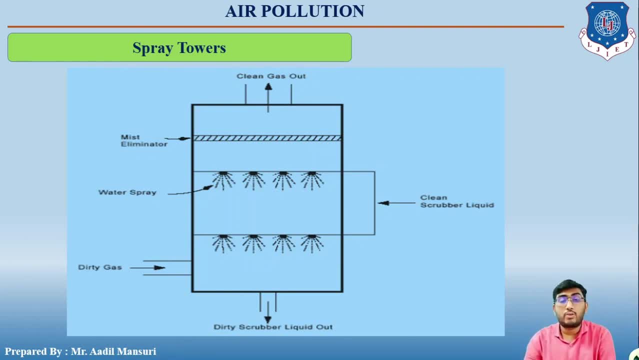 simplest type of wet scrubber is a spray tower into which water is introduced by means of spray nozzles- right you can see in the center right- and the polluted gas flows upward and the particles collected results because of dirty gas in the inertial impact and interception on the droplets. 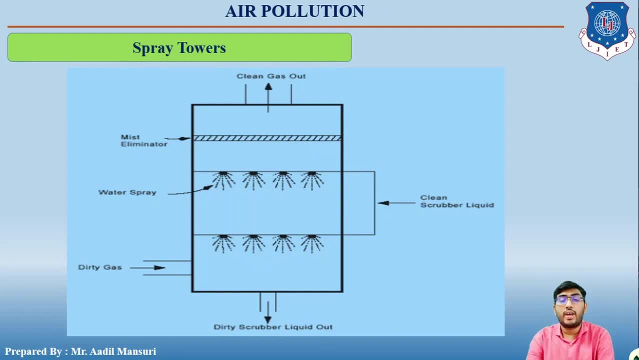 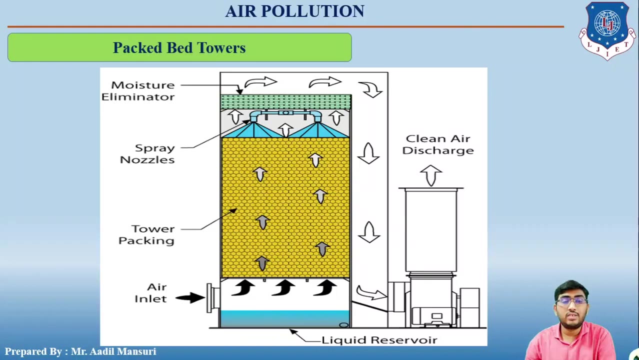 these are used for removing coarse dust where high freak efficiency is not required. they are therefore used as primary cleaners in treating blast furnace gas and for fly ash and cinder removal. okay, next is peg bed towers. so they are fiberglass packing and the polluted gas streams moves upward. 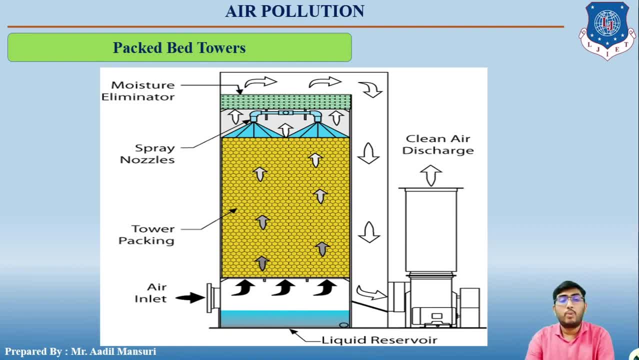 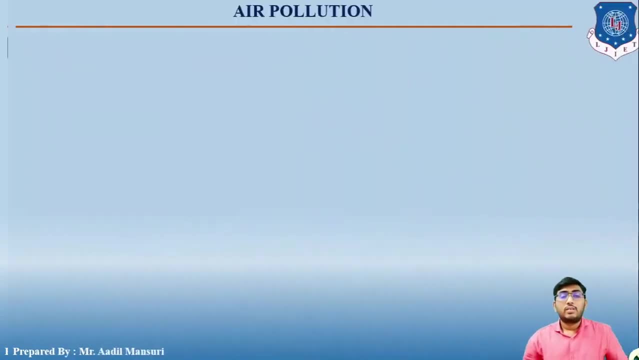 and comes in contact with the scrubbing liquid stream which is moving downwards over the packing in the film. okay, so the particles are captured by inertial compaction, while the gas stream takes a curved path through pore space of the packing. right then, talking about cyclone scrubbers, it is the modified 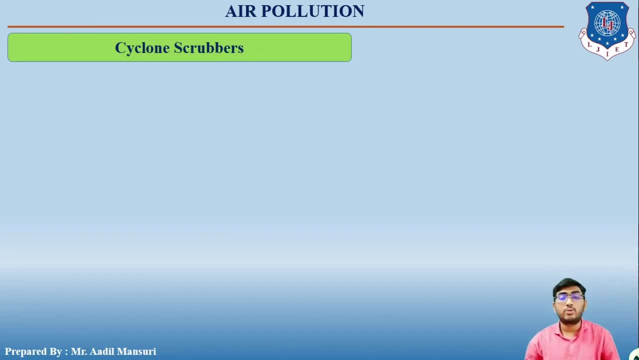 form of dry cyclone in which scrubbing liquid introduced in the gas path by spraying through the nozzle mounted on the pipe in the center of the vessel. okay, so the spinning motion is initiated by introducing the flue gas tangentially inward from the wall. okay, and the spray assists in collection of the dispersoid and tend to prevent. 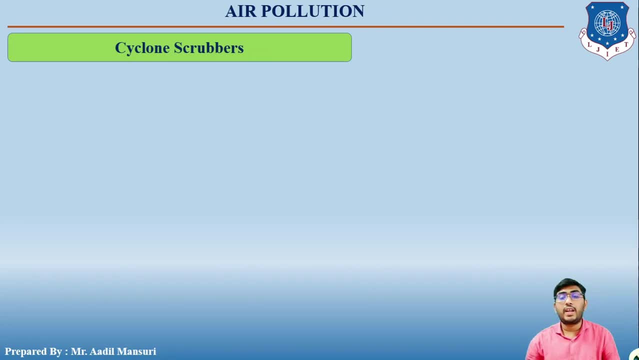 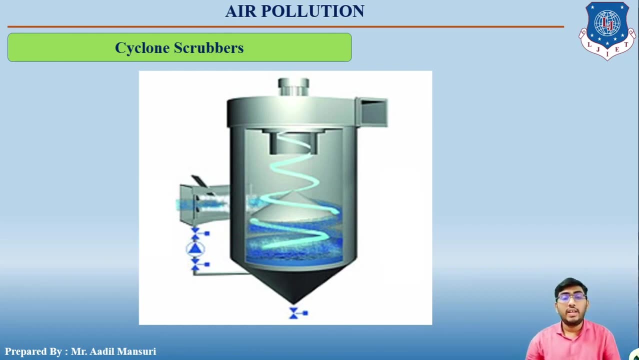 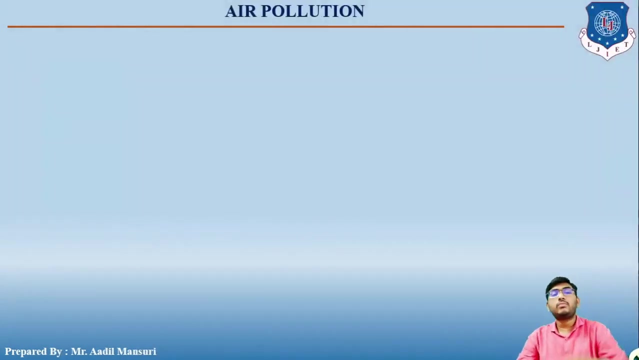 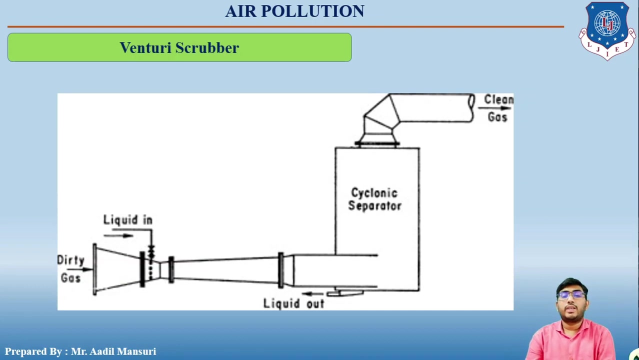 re-entrainment. the scrubbing liquid with the collected particles runs down the wall to the scrubber bottom and out, whereas the clean gas leaves through the top. okay, so you can see the picture. okay, students. so next is Venturi scrubber. okay, and after the particulates have been, fine, and after the particulates have been and the high velocity air impinges upon the liquid stream, fine, mean and after the particulates have been, distinctly Graham, this liquid is entered into the big wind line and quicklyiendo these are Yang's of fine droplets. fine, and after the particulates have been. 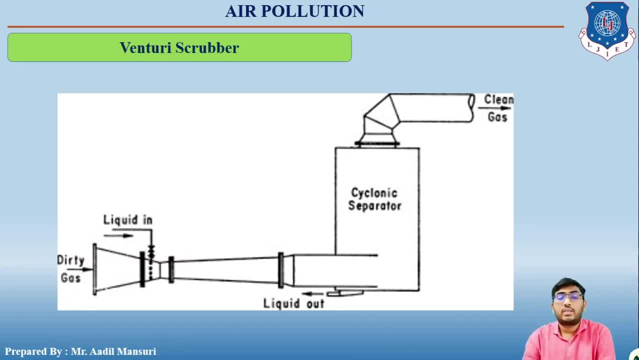 have been trapped within the liquor droplets. the resulting agglomerates are readily removed from the gas stream in the separator. okay, so such scrubbers are used in removing mists and dust from gases from pulp and paper industries and steel and chemical industries? okay, so it has. 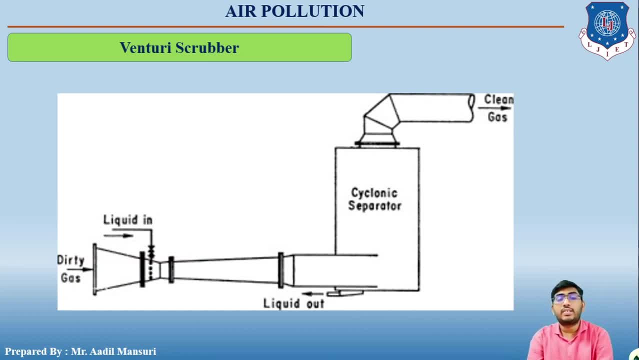 certain advantages. first, one is the simultaneous removal of gases and particulates. right two activities are carried out together: effective performance of over a wide range of loading. fine, then hazardous hazards of explosive dust, air mix are removed. hot gases can be cooled down, corrosive gases can be recovered and neutralized, and equipment occupies only a moderate space. 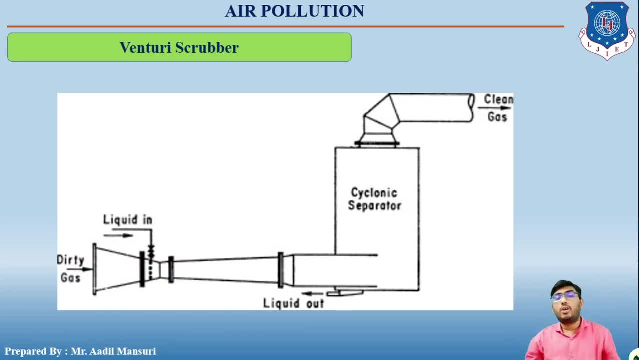 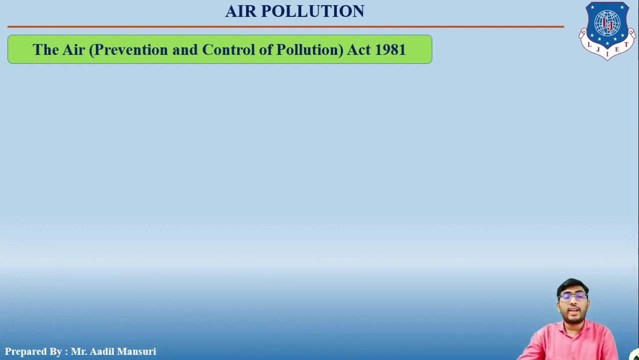 okay. so talking about disadvantages, a lot of wastewater is produced which needs disposal. fine corrosion problems is one of the disadvantage. then relatively high energy cost poses freezing problem in cold countries and very small particles, that is, submicron size, may not be captured. okay, so last is the air prevention and control of pollution act 1981. 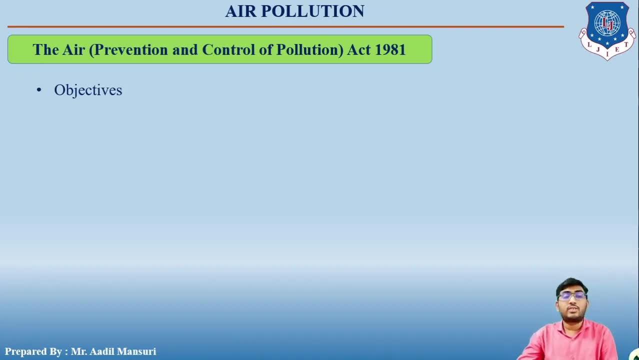 so, basically, this act consists of different objectives: constitution of the central board, function of the central board, functions of state board, powers of boards and penalties. okay, clear. so talking about what is the air pollution act. so the air prevention and control of pollution act 1981 of the government of india came into force from may 16 1981 and the 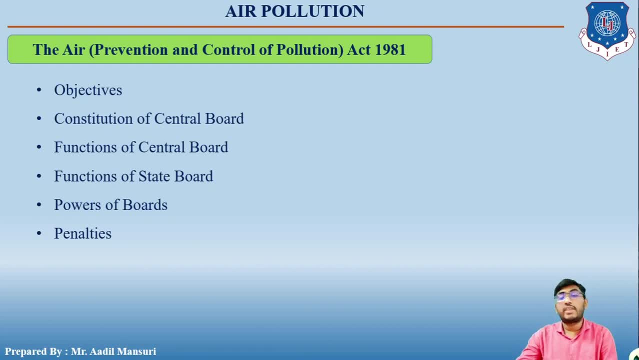 act is applicable throughout the country, unlike the earlier central water pollution act right which, for administer administering the act, the state governments have been authorized to declare, after consultation with the state boards, any area within the state uh as air pollution control area. right now, these areas may be extended, reduced uh or even merged together in course of time. pollution by. 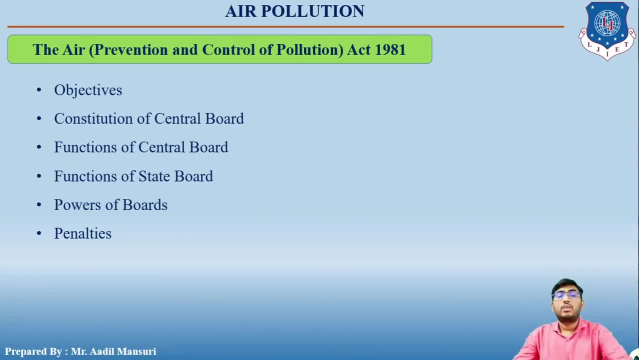 ships and aircraft is not covered by the provision. so, talking about the objectives: prevention and control and abatement of air pollution, maintaining the quality of air and establishing of boards for the prevention and control of the air pollution. so, talking about the Constitution, a state board constituted under the Act consists of different 17 members, all nominated by the state. 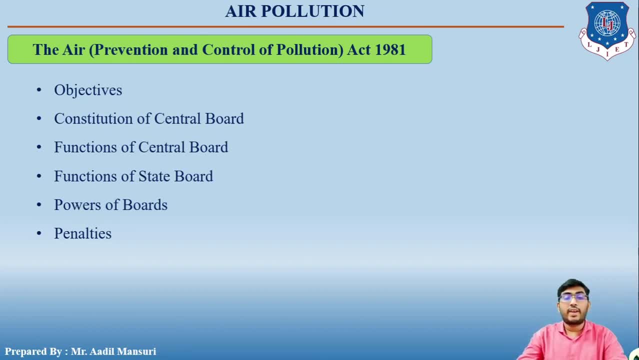 government right, which includes a full-time or part-time chairman, five official members to represent government, five persons representing the local authority, three non-official members and two person representing companies or corporations owned by state government, and one full-time member, secretary right. talking about the functions, who, then? there are several. 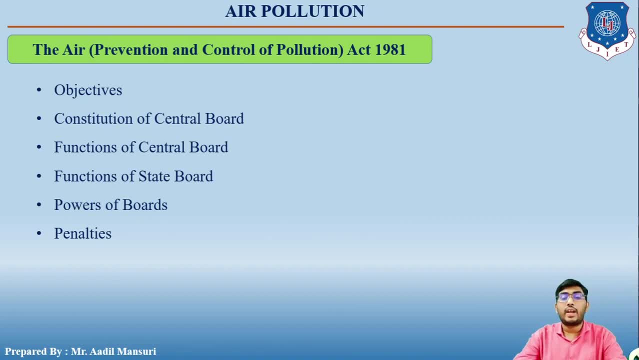 functions like to improve the quality of the air. to prevent and control and abet the air pollution in the country. to advise the central government on any matter concerning the improvement of the quality of air. then to plan and execute the nationwide program for the prevention, control and abatement of the air pollution. then to control the 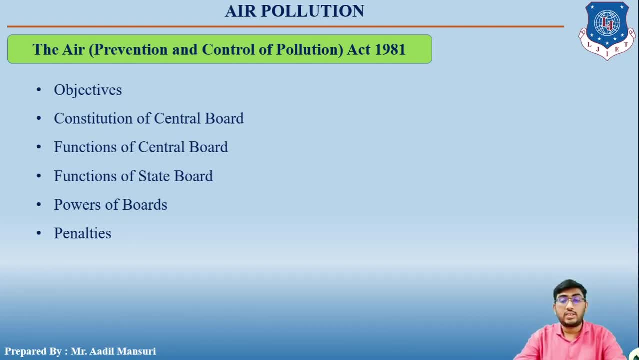 activities of the state board, provide technical assistance and carry out research relating to the prevention and control of the air pollution. okay, then, to lay down standards for quality of air and, last, to establish the or recognize the testing laboratory. so these were the functions of the central board. now,